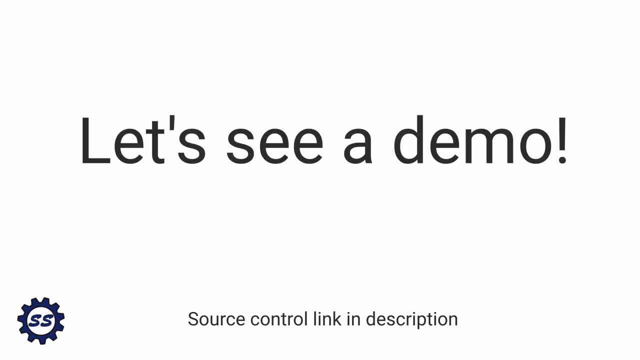 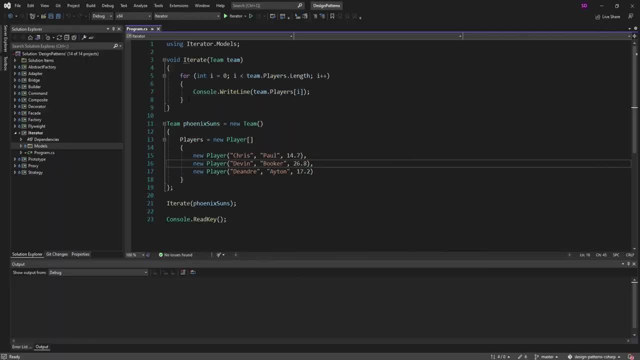 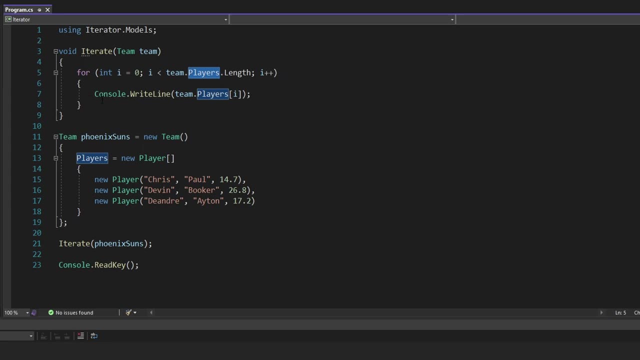 uses that iterator to traverse the collection. So in this demo we are going to leverage the iterator pattern to traverse various different collections. So here in this demo I have this iterate function and this takes in a team And a team has players that we iterate over in this. 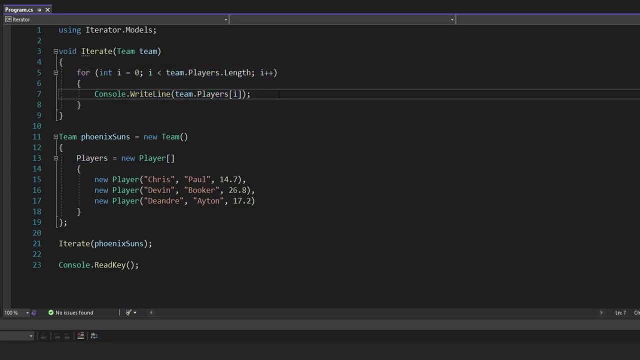 for loop and we simply write out each player on the team to the console. So, digging into this, let's look at team again that simply has an array of players and then if we look at player that simply has a first name, last name and points per game and we write that out to the 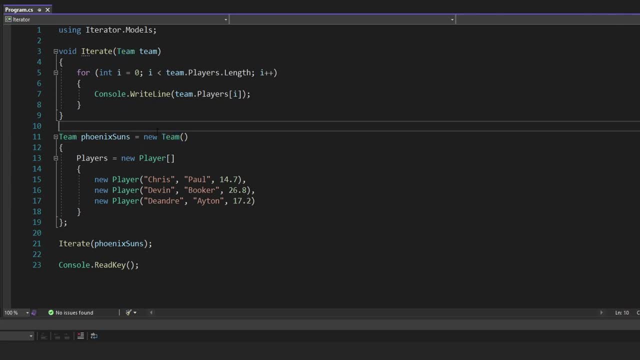 console. So back up to the programcs, where we put this all together. we initialize this team, that is the for loop, And we also have a team that simply has a players name And again, if This is the Phoenix Sun, so kind of dealing with basketball here. 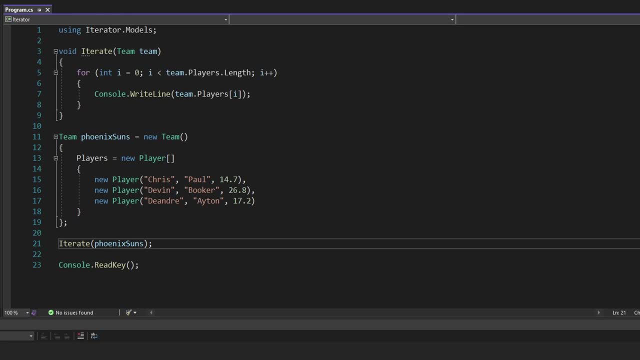 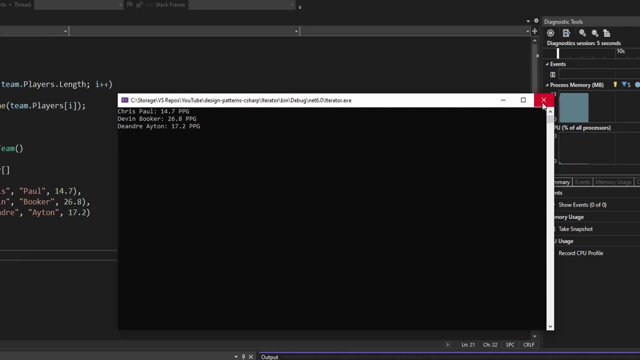 And then we simply iterate over this team and write out each player to the console. So let's run this and see it in action. There we go, simply write out these three players. I didn't put the whole team, just three for an example. 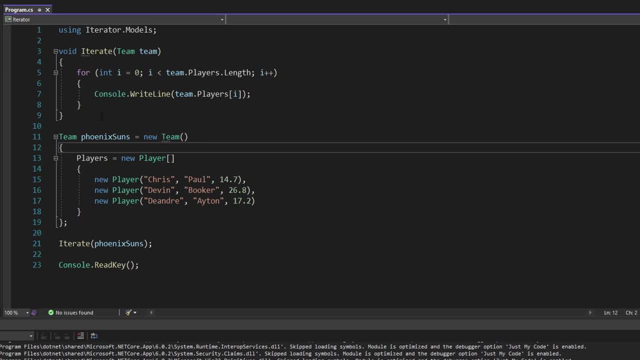 So the problem we have here that we're going to solve with the iterator pattern is that I want this iterate function to support other collections too, not just team. I want it to support another collection that also has a collection of players inside of it. 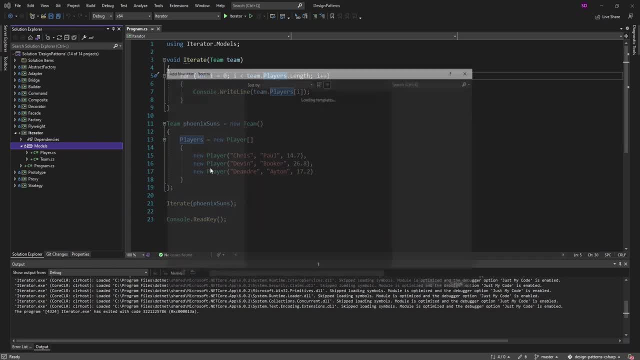 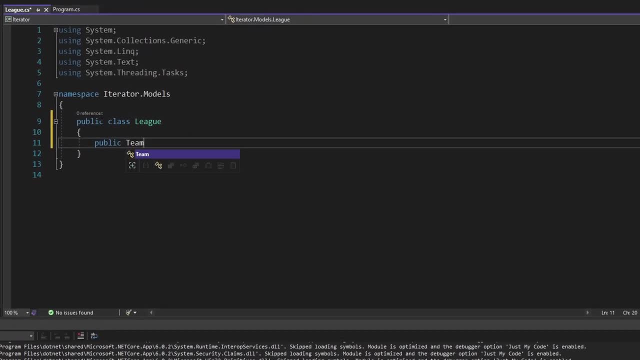 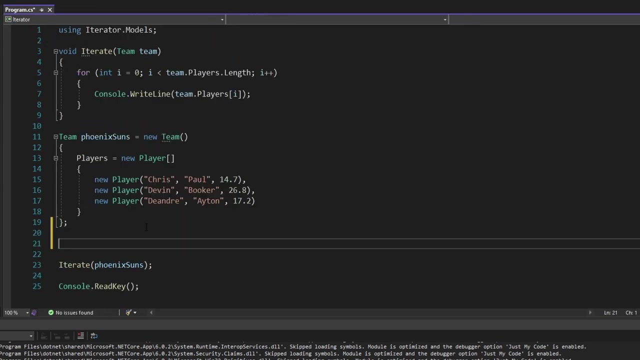 So, for example, let me add another class over here And this is going to represent the entire league. So we'll call it league And the league is just going to have a collection of teams, So just an array of teams. So now back in our programcs. let's initialize our league. 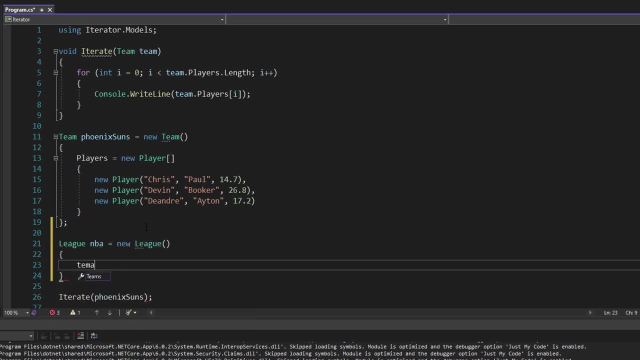 And this is the NBA dealing with basketball again, And let's pass in all of our teams to the league. So a new array of teams, And right now we just have the Phoenix Sun, And let me add another team too, just to enhance this demo. 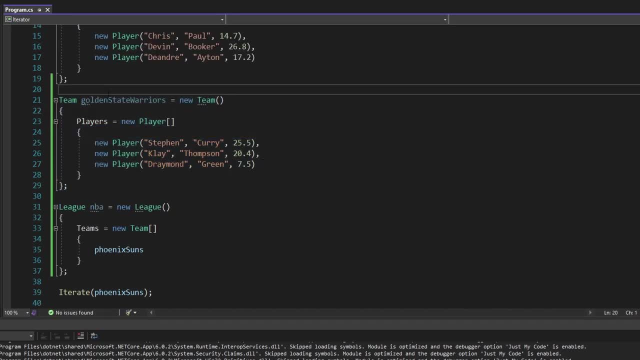 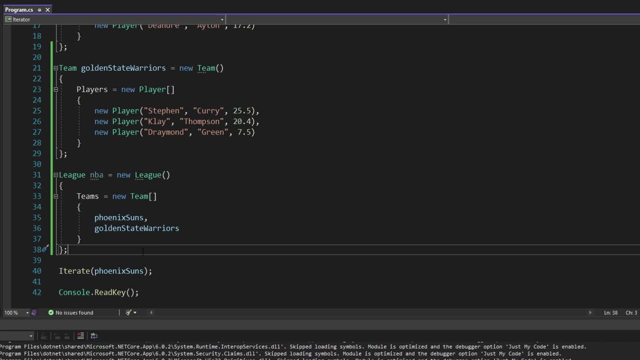 And I'll just grab this off camera real quick. There we go. added the Golden State Warriors as another team. Let me put that in our league. So add that to our team's collection. And now getting back to the problem that we want to solve with the iterator pattern, 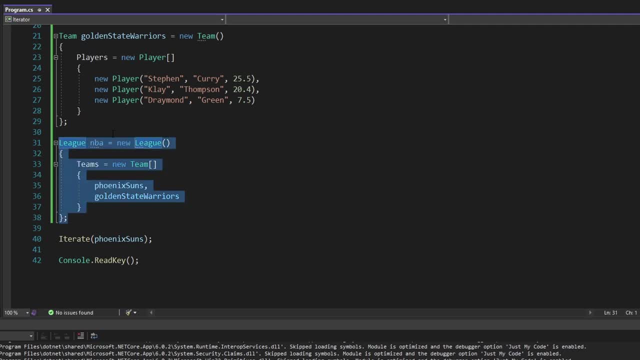 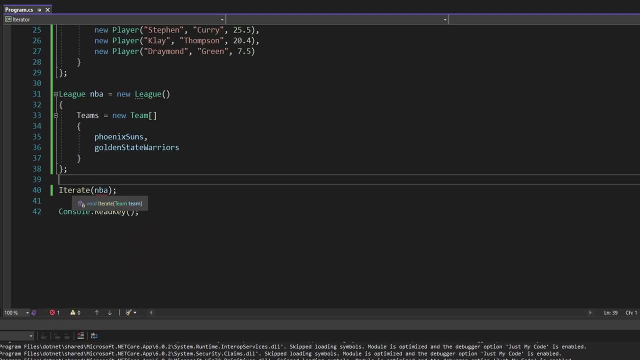 So ultimately, I want to iterate over all of the players in our league. So really I want to pass the NBA to this iterate function, But at the moment we can't do that because this iterate function expects a team to be passed in. 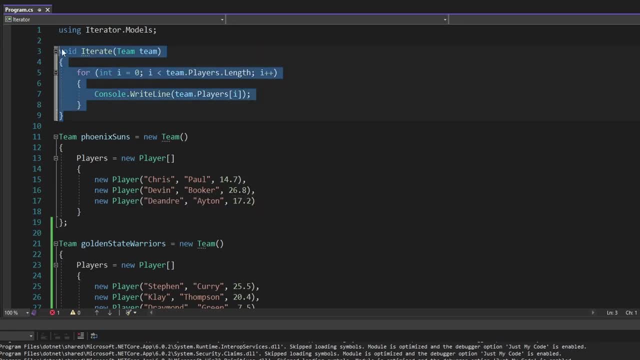 So, ultimately, what we need to do is we need to update this iterate function to be able to take in either a team or a league, And then the iterate function can get an iterator for whatever object- either a team or a league- that gets passed into this function. 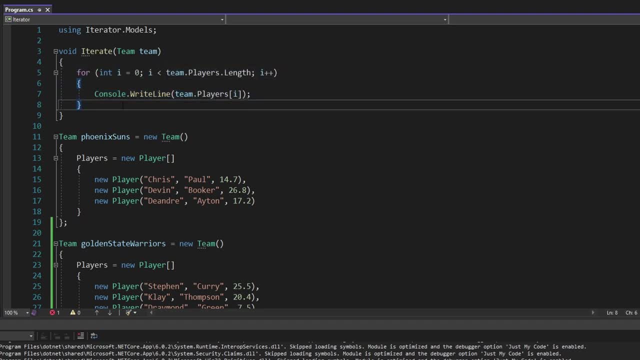 And then use that iterator to iterate over the collection of players. So if we want to pass in either a team or a league to this iterate function, then this function is going to have to depend on some kind of interface that team and league implement. 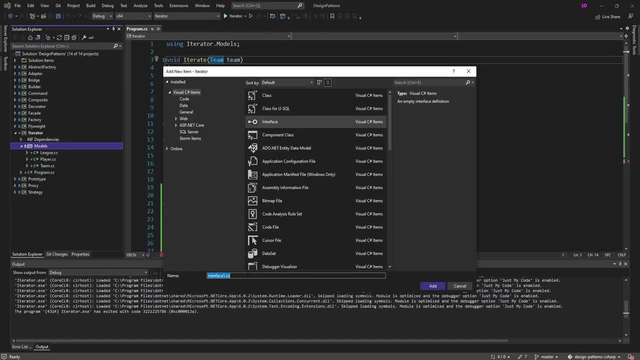 So let's create that interface that we can depend on, And really what this iterate function wants to do is iterate over a collection of players, So we'll call this interface an iPlayerCollection. So now that we have this interface, we haven't really done anything with it. 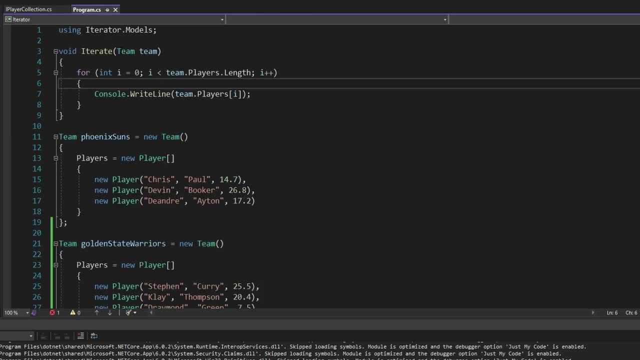 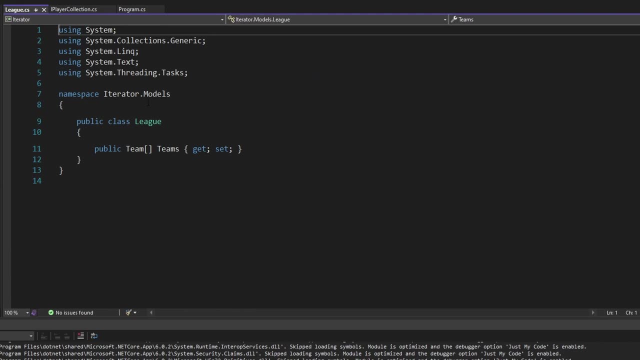 but let's use it and depend on it. So this iterate function is going to get a iPlayerCollection passed in, So let's reference that, And then our league is going to implement the iPlayerCollection interface as well as the team class. 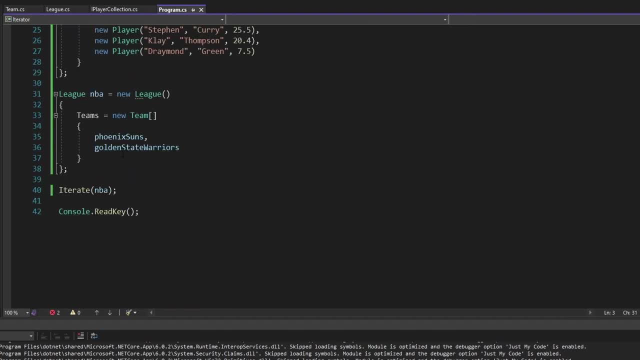 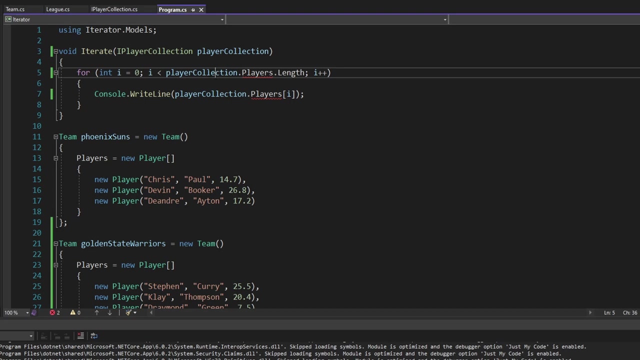 So now if we go back to our programcs, we can successfully pass in our league of NBA as well as either of our teams There. we go, no issues there. But now, if we get into this iterate function, we're trying to access the player's property on an iPlayerCollection. 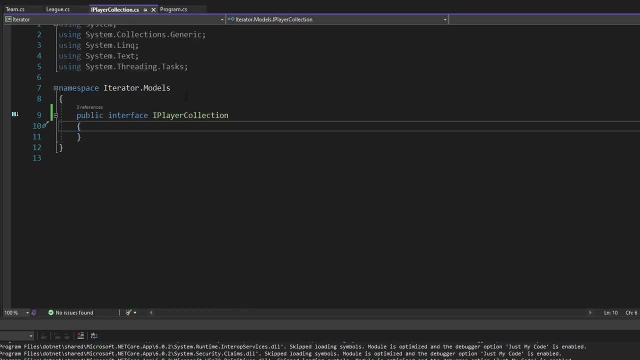 which obviously doesn't exist. So we might be tempted to add that player's array to the iPlayerCollection. but we can't do that because even though our team class has an array of players, our league class doesn't: it has an array of teams. 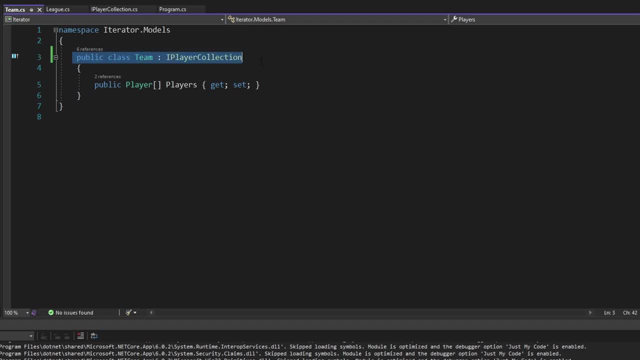 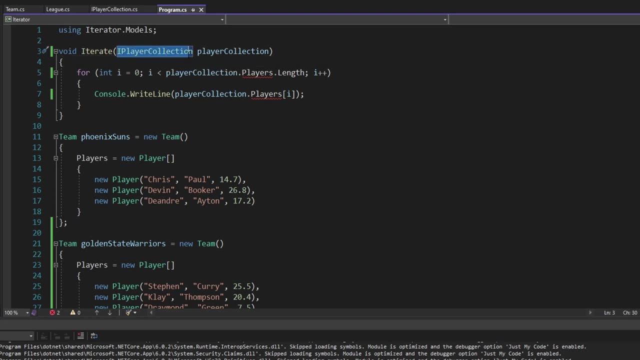 So our league class and our team class are going to have to be traversed quite differently in this iterate function. So really, all this iterate function can do is ask the collection: how do I traverse you? So in other words, the iterate function is going to get back an iterator from the player collection. 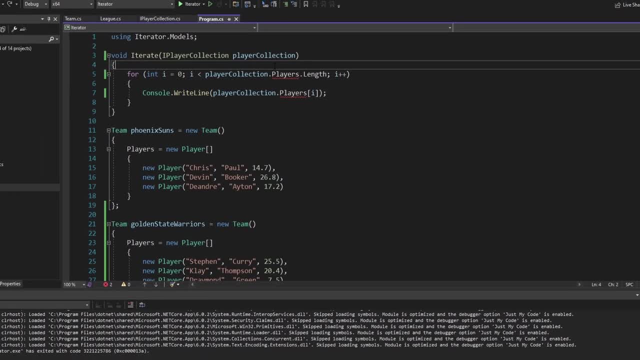 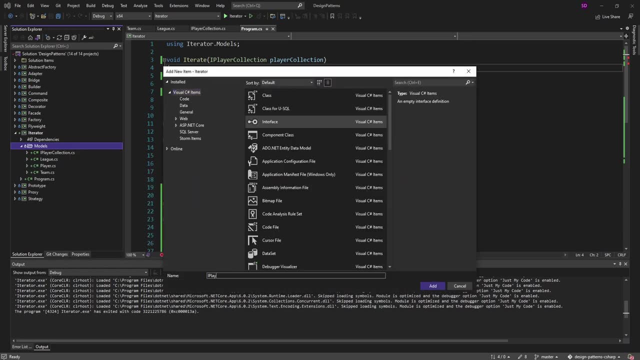 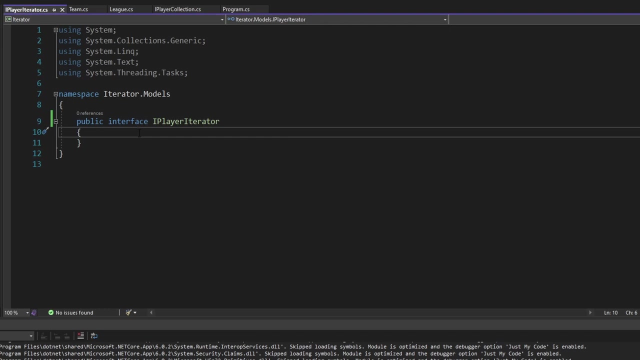 that the iterate function can use to traverse the player collection. So let's create an interface for our various iterators that we're going to have to create. We can just call this the iPlayerIterator. So the iterate function is going to use a player iterator to traverse through whatever collection it has. 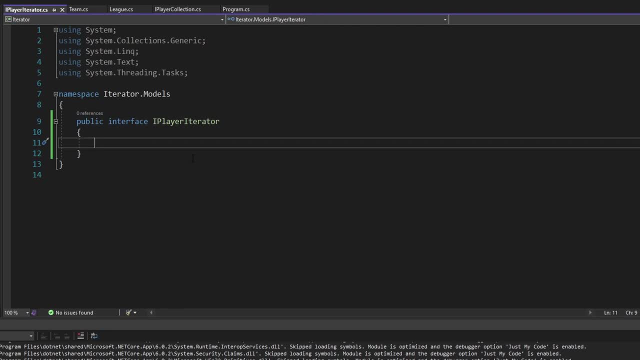 So it's going to need some helper functions to do that. It's going to need a way to tell the iterator to go to the first player, So this can just be a void function called first. It's also going to have to tell the iterator. 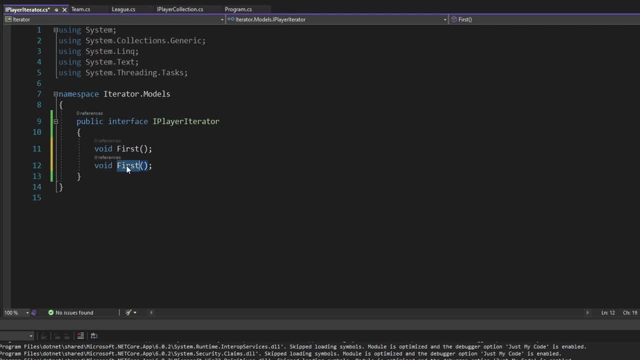 it's also going to have to tell the iterator to go to the next player, So this can just be next. It's also going to have to ask the iterator if there's any other players left to traverse, So this can just be a bool for has next. So if it. 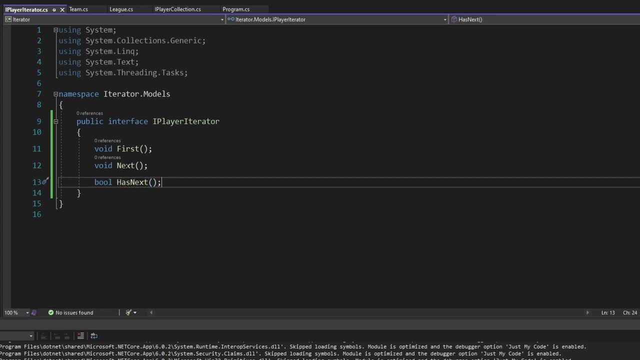 does have more players to traverse, this will return true, Otherwise it'll return false. And then, finally, we're going to have to get the current player that the iterator references, So this can just be current. So, now that we've defined the player iterator, we're going to have 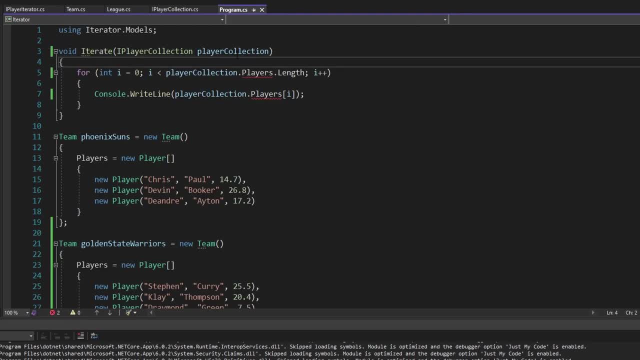 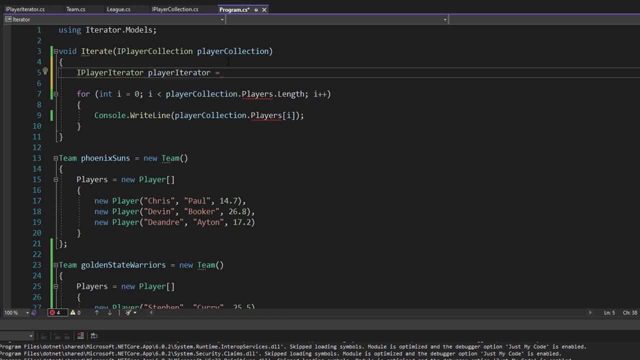 to get it. And the way we get the player iterator is asking the collection to provide it. So this iterate function is going to get an iPlayerIterator by asking whatever player collection it has to create one. So we can just add a function to iPlayerCollection called createPlayerIterator. 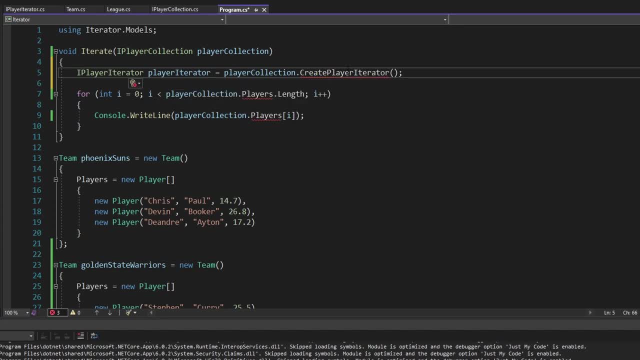 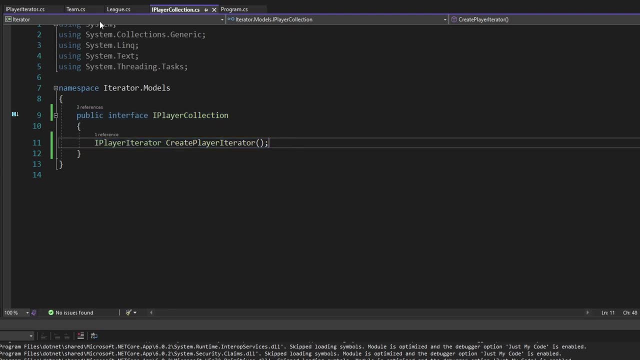 So we're going to have to generate that on our iPlayerCollection interface. So there we go. That's generated now. So now that our iPlayerCollection interface has this function, our team and lead classes are going to have to implement it. So let's start off. 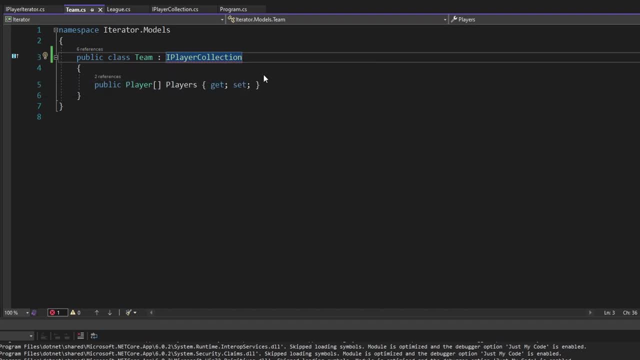 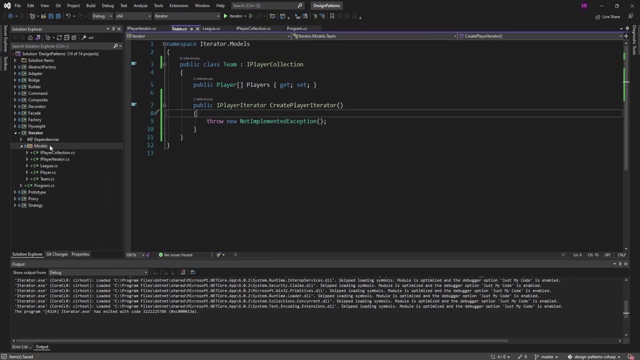 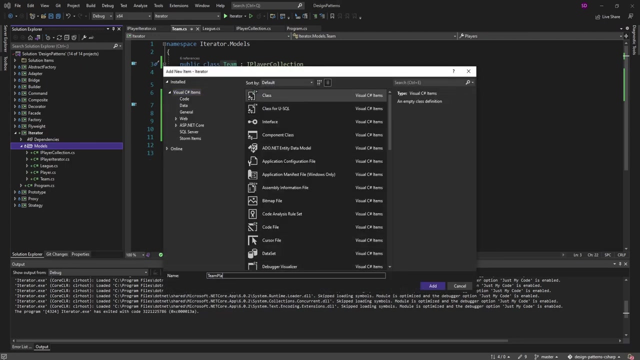 with team. Let's implement the create player iterator function And of course, this is going to have to return some kind of iterator. So let's implement an iterator that'll be used for this team class. So let's add a new item here. We'll call this the team player iterator And let's 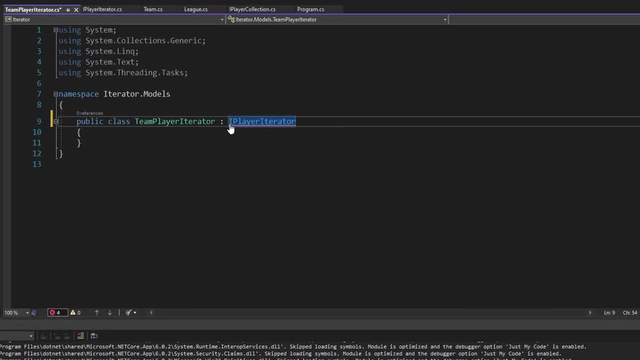 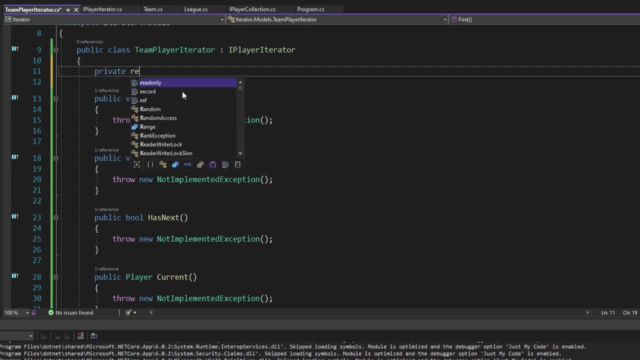 implement our I player iterator interface here And if we want to iterate over a team first, we're gonna have to actually get the team passed into our iterator. So let's do that. We're gonna have a read only field for the team we want to iterate And we can just get that passed through. 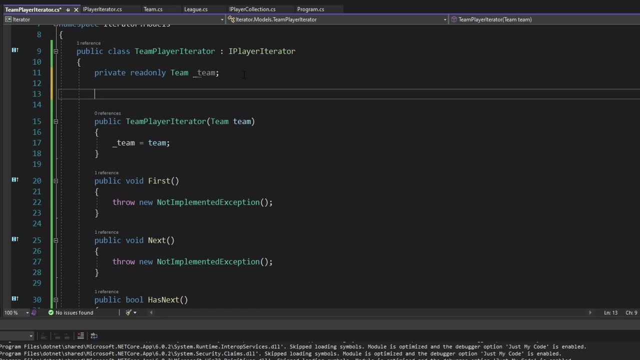 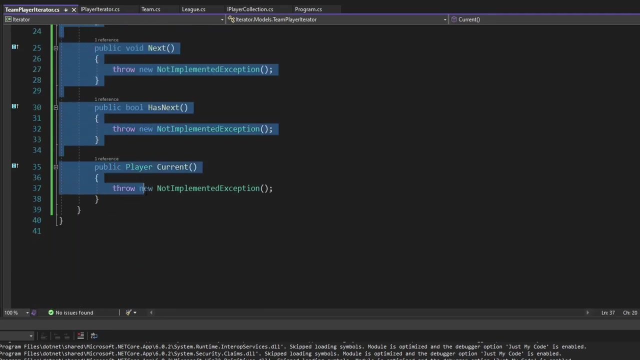 the constructor. So another thing we're going to need is the current position we are in traversing the team. So we can just track that with an integer for the current index we're at with our iteration. So we just call this current index And with that implementing these other methods makes more sense. So first, 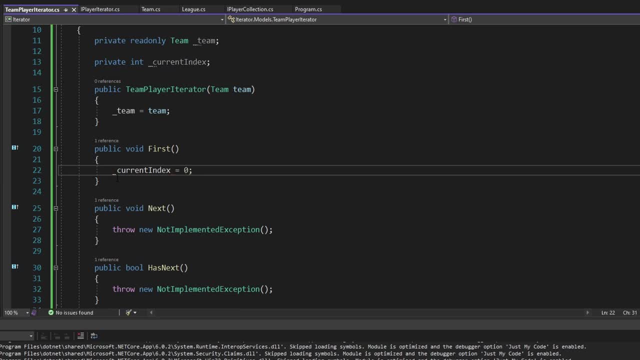 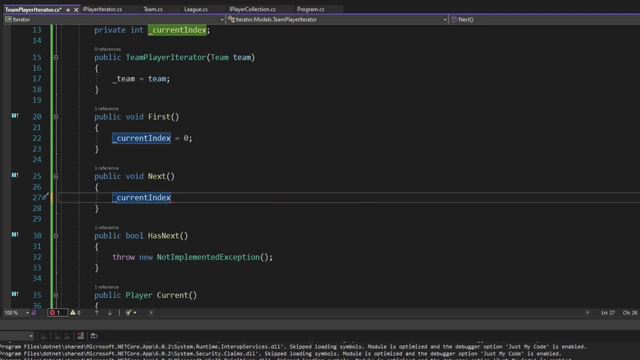 of course we're going to set the current index to zero. So basically setting the iterator to the beginning And then next is going to increment the current index, So we can just do a plus, plus, Then for has. next we want to compare against the length of our player's array. So we want to check. 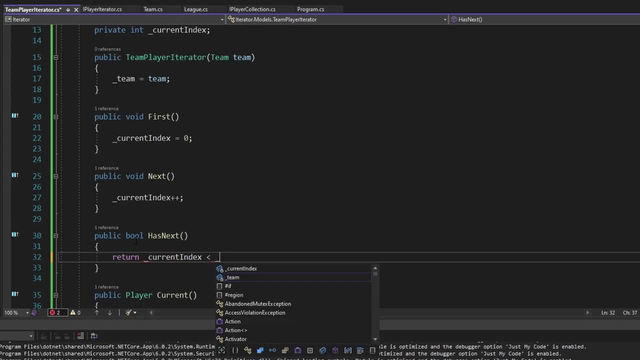 if the current index is less than our player's array length. So we'll take our team player's array length And we also want to subtract one from this, because if we were just one less than our player's array length, then that means we're at the end of the array and we actually do not. 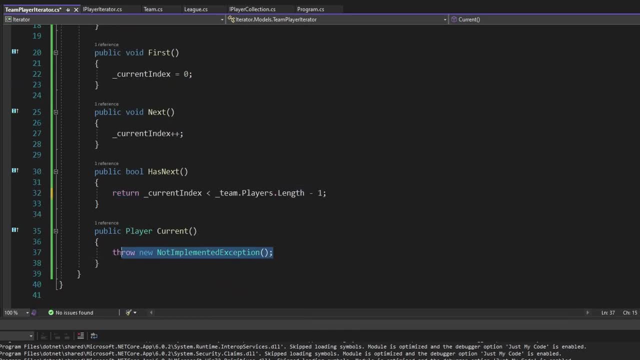 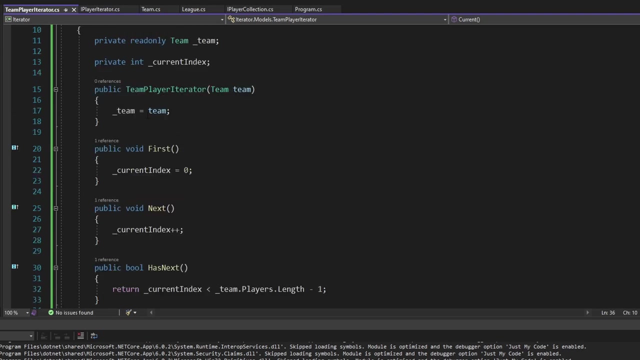 have a next. So this minus one is quite important. And then finally, bringing it all together, current will just return the current index on the player's array. So just pass in current index there And our iterator should be working as expected. So I do want to test this out where we are right. 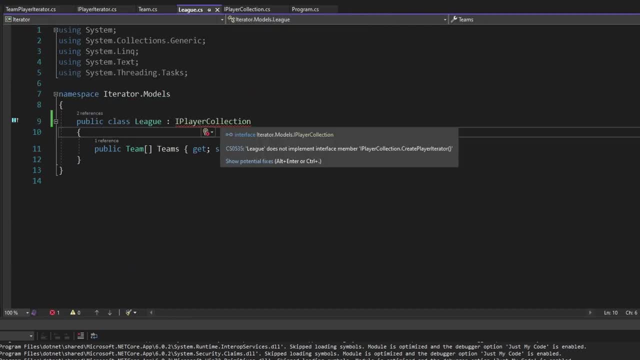 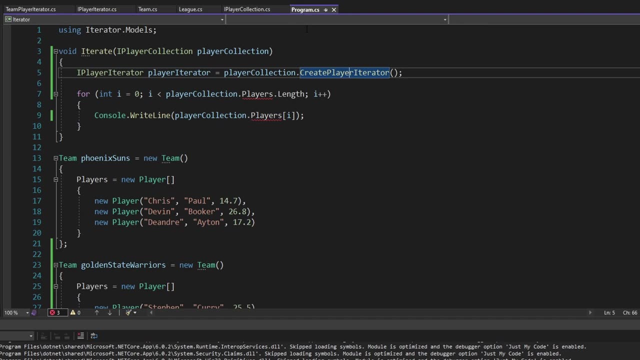 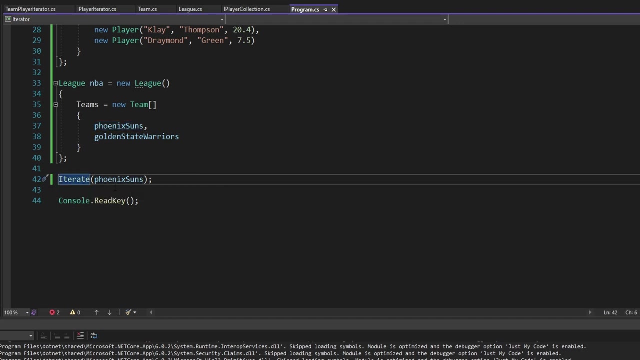 now. So I'm just going to not implement the I player collection on our league at the moment. So there we go, just commenting that out. And now, if we go back to our programcs, we're just going to pass in our team to this iterate function, since that implements our I player collection interface. 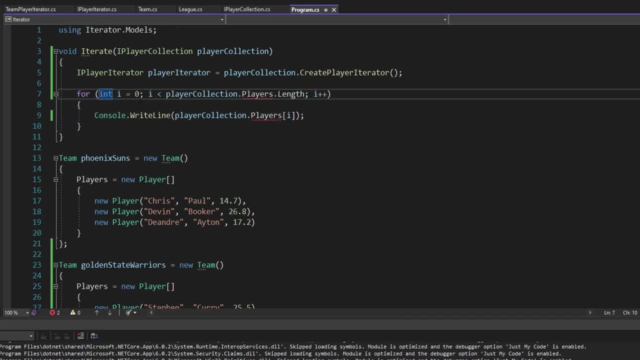 And now let's use our player iterator in this for loop. So the first thing we want to do is tell our player iterator to go to the first item, And then we only want to continue with our iterator if our player iterator has a next value. And then, finally, after each loop, we want to tell: 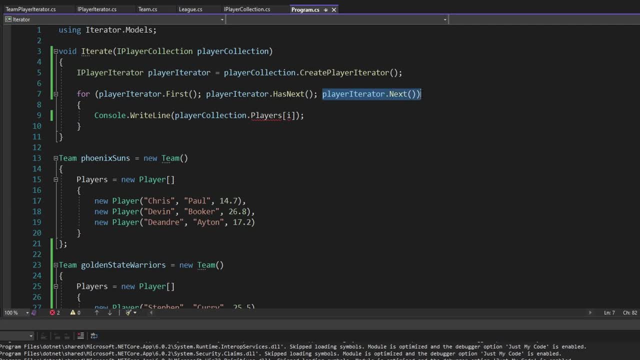 our iterator to go to the next item. So we'll call player iterator dot next, And then if we want to write out the current player, we can just use our player iterator again and get the current item. So now, if we try this out, we should write out our three players, And we actually don't. 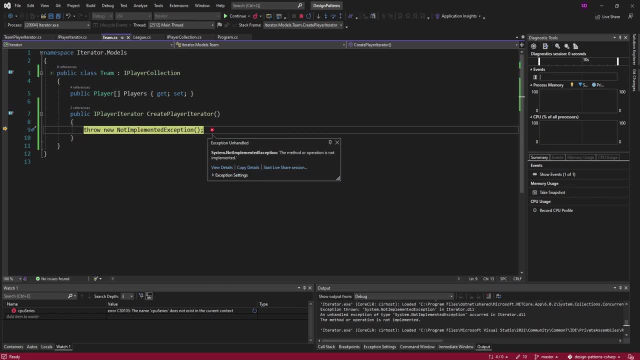 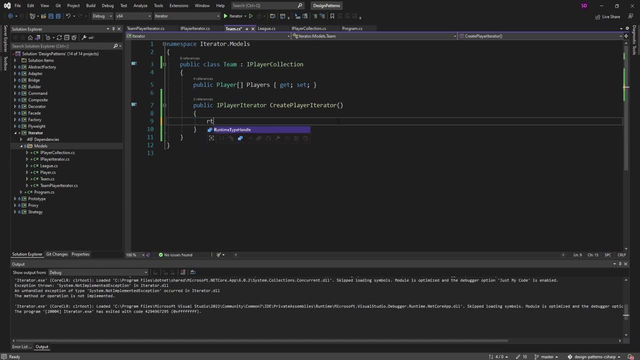 because I forgot to use our team player iterator in our team class. So right now we just have this not implemented exception. But what we want to do is return a new team player iterator and pass in this team, which is just literally this And looks like we only get two players written. So this is. 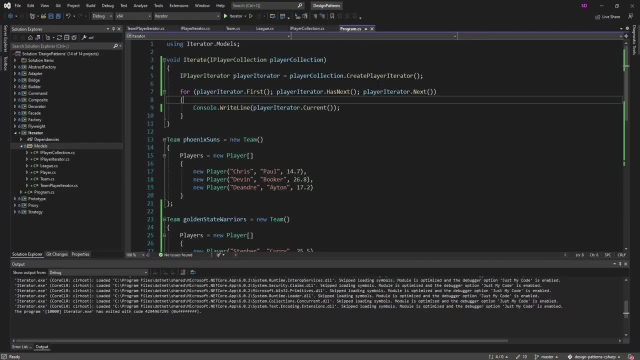 probably a problem with our has next check. So what happens in our for loop is: at the end of our second to last iteration we call player iterator dot next, which puts our iterator at the last item. But then we check has next And at this point, since we are on the last item, has next returns false and we end up not. 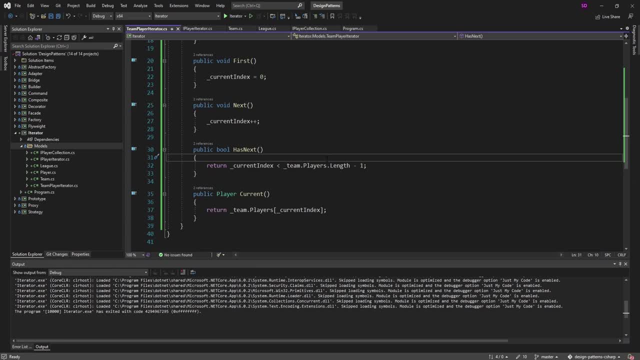 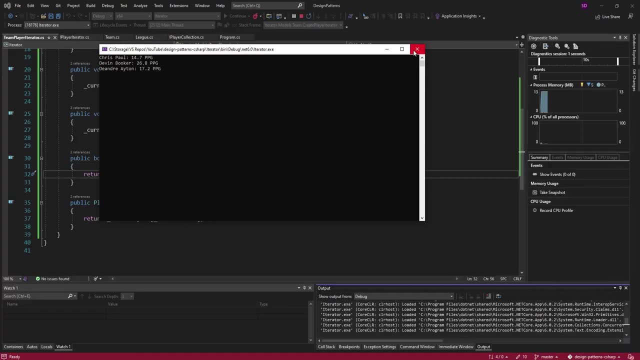 printing out the last item. So really all we have to do is go back and not do this minus one check. So let's remove that And this should all work now. So there we go, we print all three players and no errors, of course, But then has next isn't really describing what's happening. 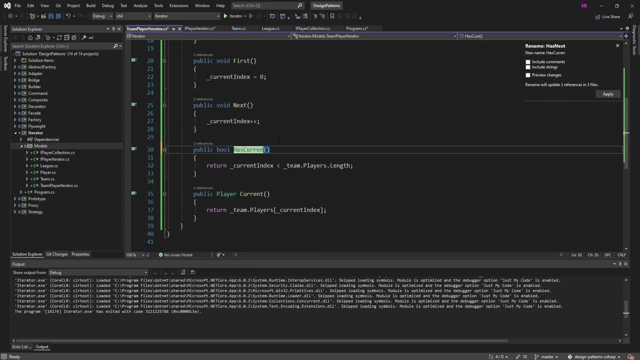 Here Instead. this is really has current, So we can rename that there, And I've even seen some iterator implementations have some kind of is done method instead. then in their for loop they'll check the iterator is not done, And I almost feel like that's more common, So I'm going to do that. 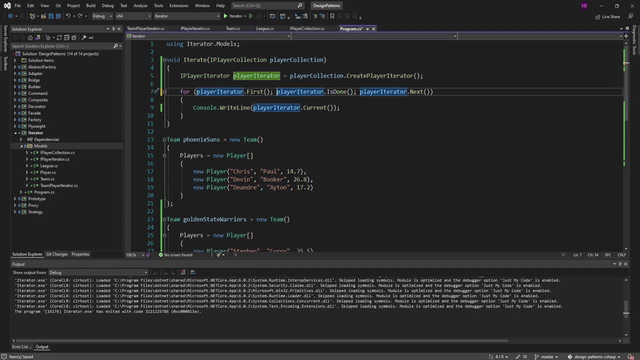 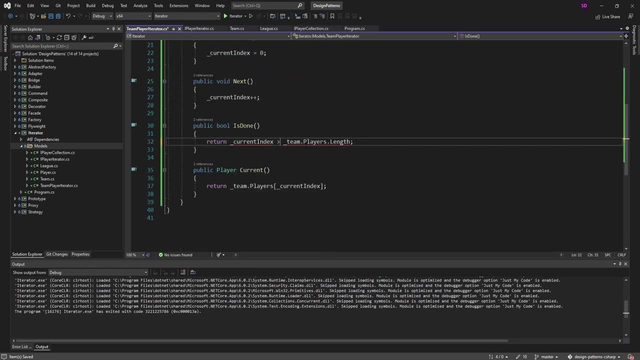 here Let's make this is done. And we want to check if the player iterator is not done. So there we go with the exclamation point And then we are done if the current index is greater than or equal to the array length. So let's try this. 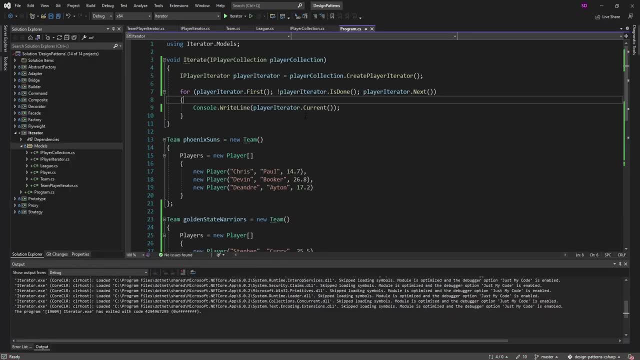 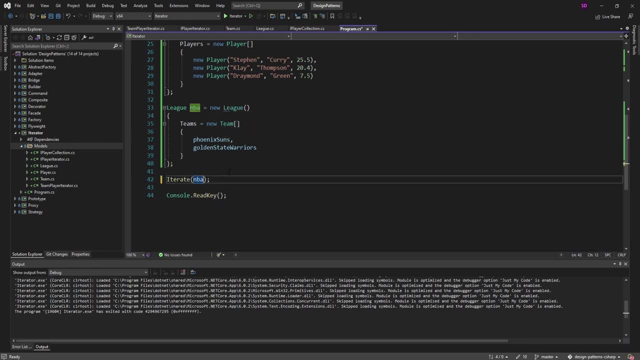 Again. now there we go, we still get all three players printed. So now, getting back to our main goal, I want to print all the players in our league. So let's pass in our league to the iterate function. But league at the moment does not implement I player collection. let's bring that. 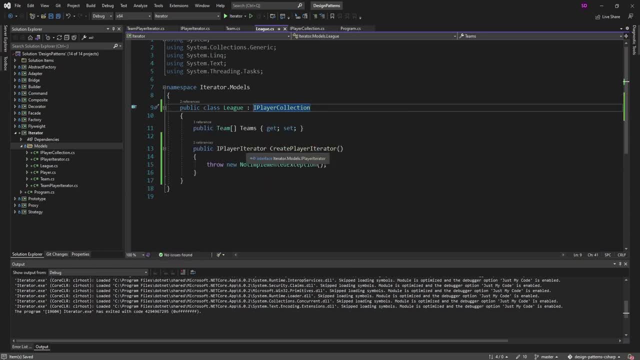 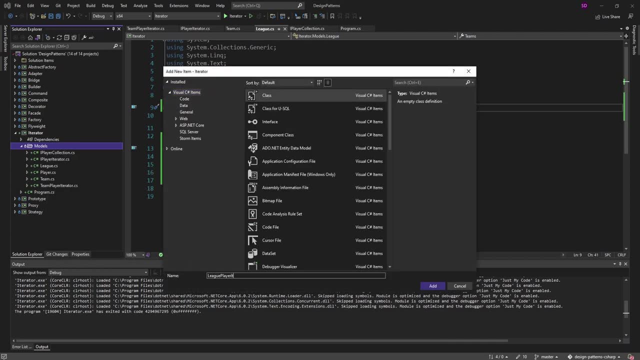 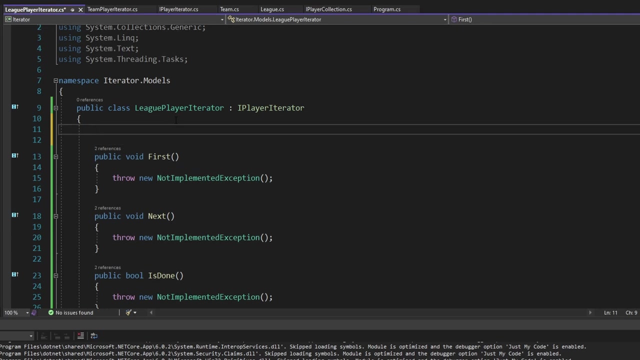 back and implement that interface, which means we're going to need some kind of league player iterator. So let's add that- a new class for a league player iterator. this will implement I player iterator. So let's implement that interface, So similar to the team player iterator we're going to need our 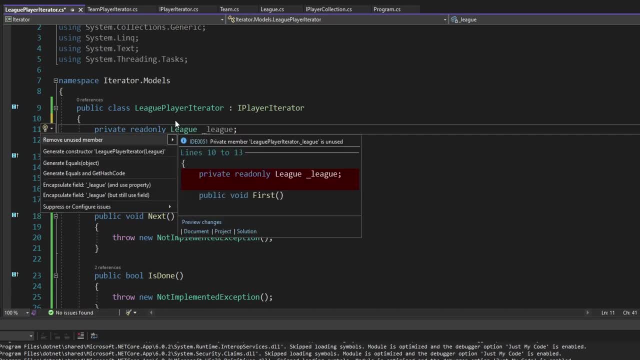 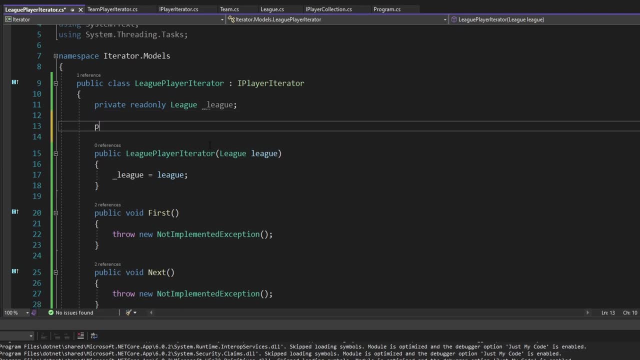 league passed in to the iterator. let's generate a constructor for that, And this iterator is going to be a bit more complex. So, similar to the other iterator, we're gonna have to track which team we're currently iterating over, So we can have a current team index And then in this iterator, 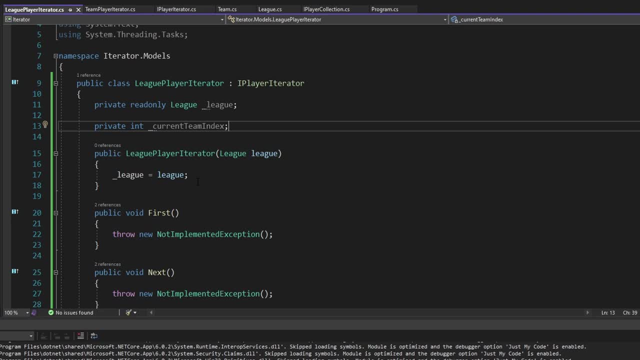 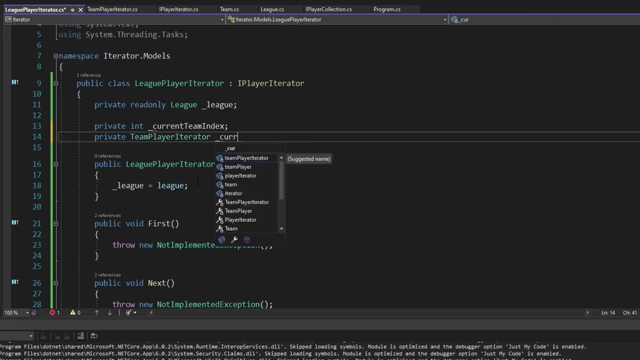 we're also going to be iterating over all the players in a team. So, that being said, we can use our team player iterator inside this iterator as well. So we're going to reference the current team player iterator And we'll keep this up to date, depending on which team we're currently iterating. 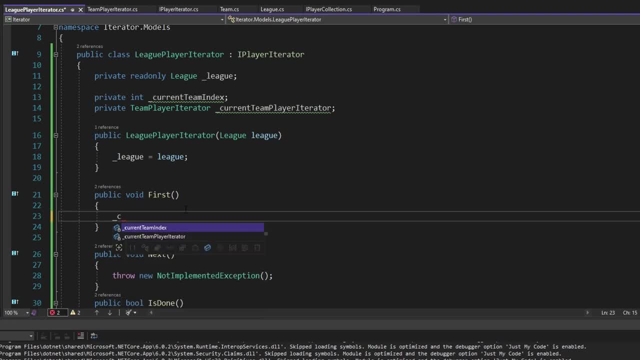 over. So, starting off with, first, of course, we want to set the current team index to zero, So setting the iterator to the beginning, and then we want to set the current team player iterator to a new team player iterator, passing in the current team that we're on, So getting into our 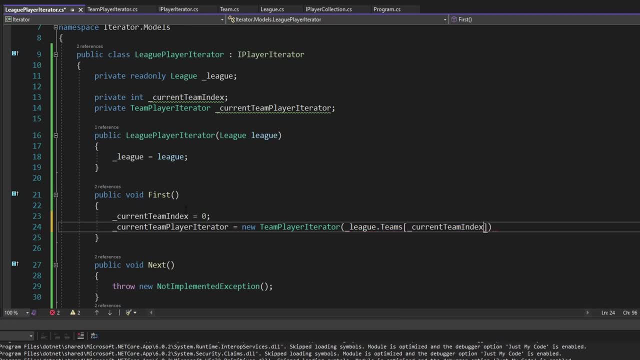 teams array And passing in the current team index, which is zero, So starting off with the first team. but at this point we have to be careful Because if our teams array had zero teams in it, then this would give us an index out of bounds exception. So we just have a check here to make. 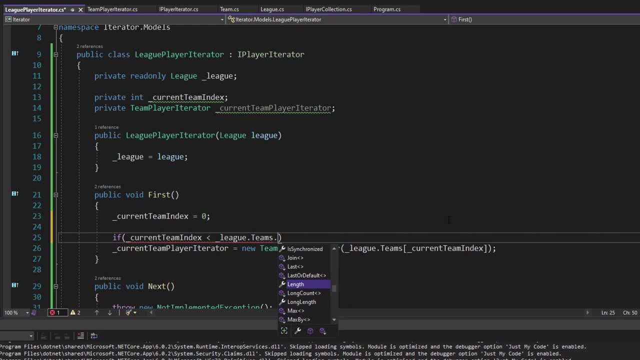 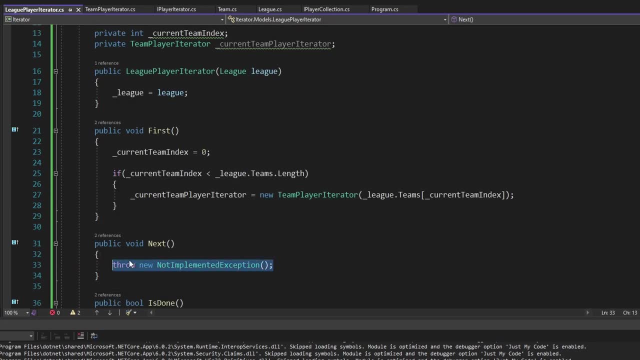 sure the current team index is less than the amount of teams in our array, And if it is, then we can initialize this iterator. So now, moving on to next. this will be a little bit more complicated too. So, starting off, our current team player iterator could be null if we didn't initialize it here. 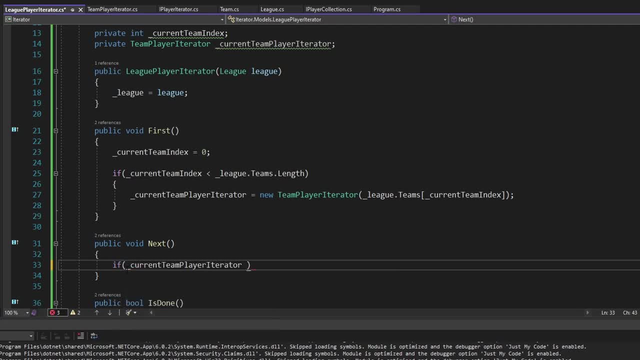 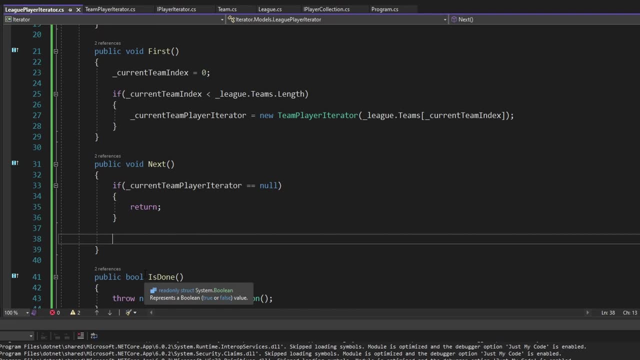 So let's add a little null check here to make sure that if it is null then we just return early from this function and do nothing. But then if we actually have an iterator, then we can take that and call next. But then we have to account for if this iterator is done. 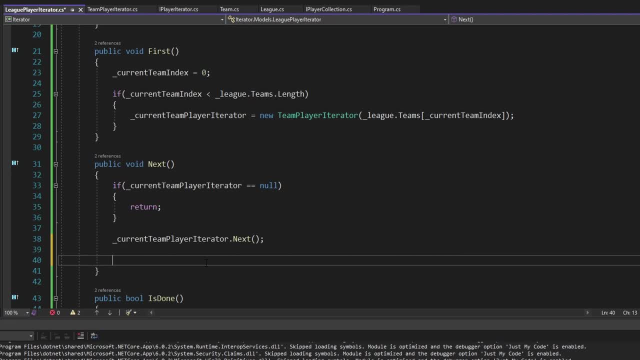 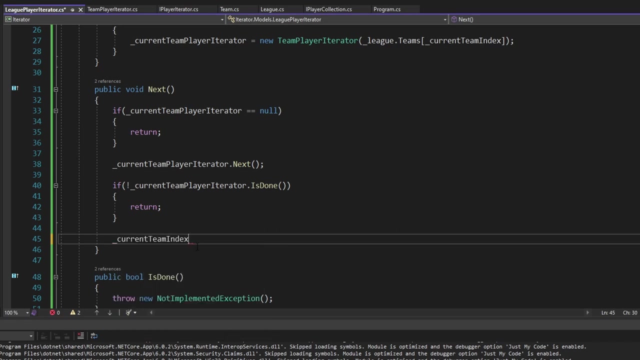 then we want to move on to the next team and create an iterator for that. So first let's check if the current team player iterator is not done, Because if it's not done then we can just return out of this function and keep on going with our iteration. But if it is done then we want to move on to the next team. 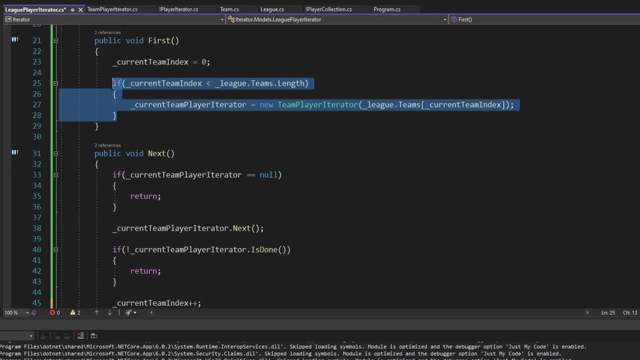 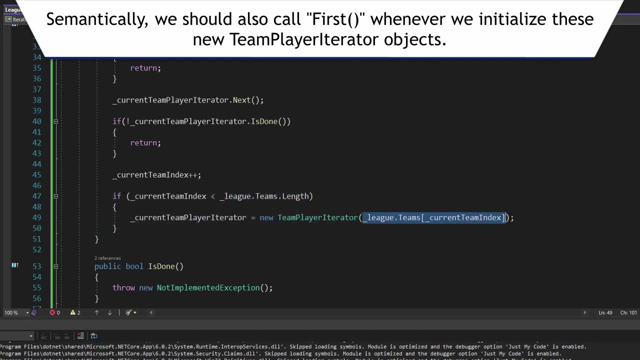 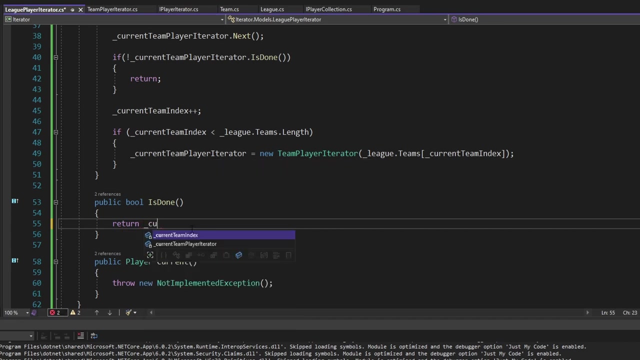 So increment that index and then initialize another iterator for the team that we're on. So same thing as before: got to have this guard as well. So we don't go out of bounds on this array. So is done. same kind of thing. we're gonna have to check if the iterator is null, Because if it is, 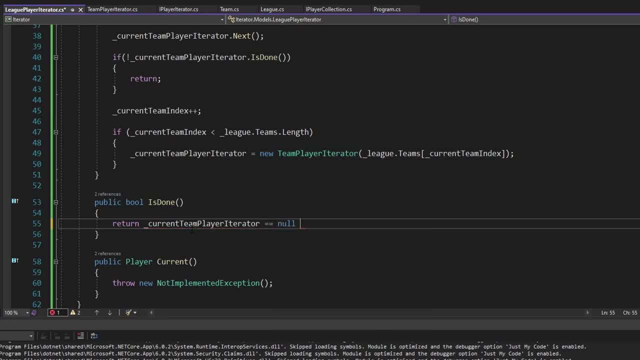 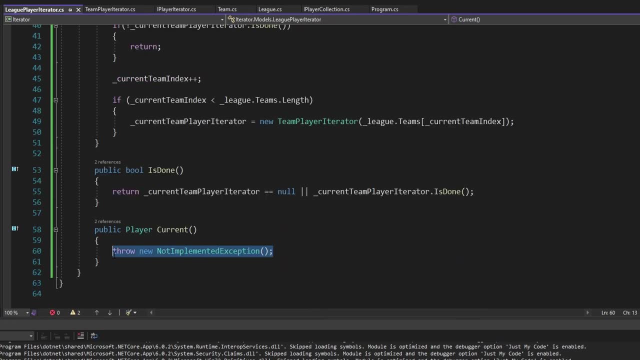 then that means we're done with our iteration. But then if it's not null, then we can delegate to the current team player iterator and check if that's done. And then, finally, for current- this one is straightforward- we can just dig straight into our current iterator and get the 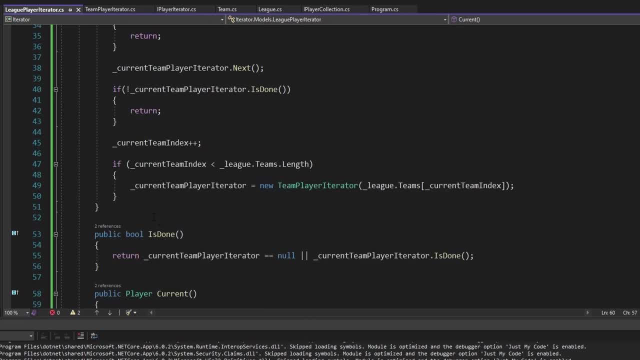 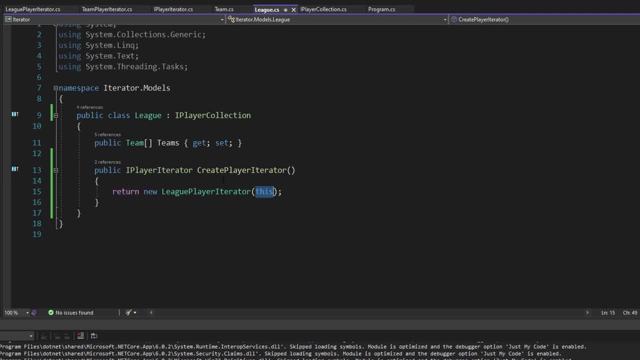 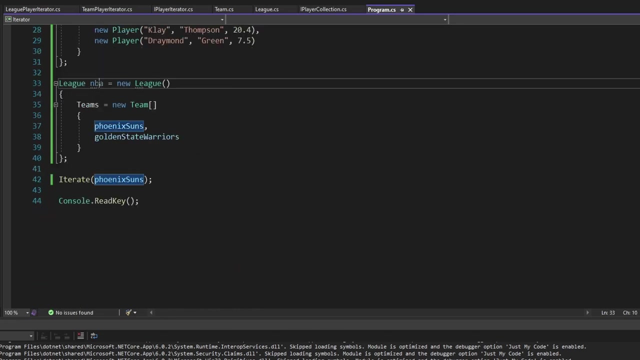 current value. So now this iterator- a little bit more complex for sure, But getting into our league, let's make sure we return this new iterator and pass in this current league instance. So now back in our programcss. our league is ready to print out, So let's pass that into our iterate function. 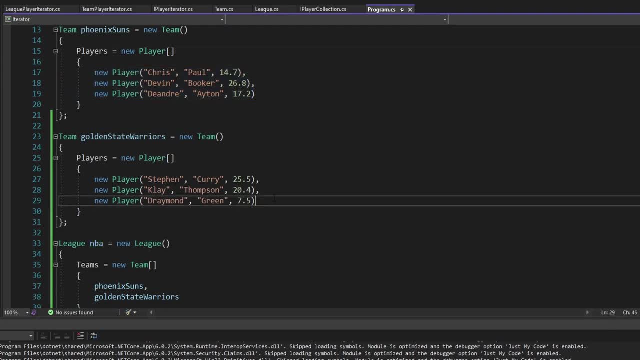 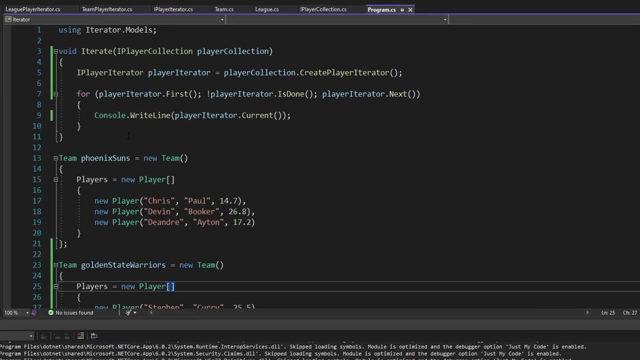 There we go, And we should get all of the players in our league printed out to the console. So here we go, And there we go works just as expected. So with that we've now implemented the iterator pattern from scratch. So our iterate function now takes in an I player collection, which could be: 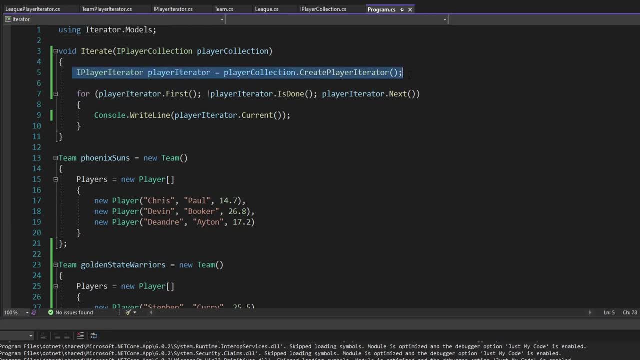 either a team or a league, But whichever one we have. this function asks the player collection to get back some kind of iterator, And then it uses that iterator to iterate through the players in either the team or the league. So whenever the player collection is a 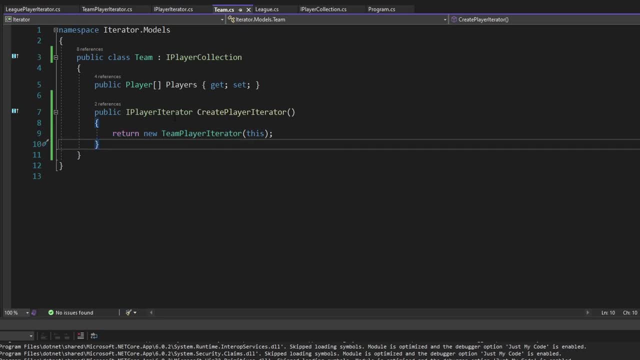 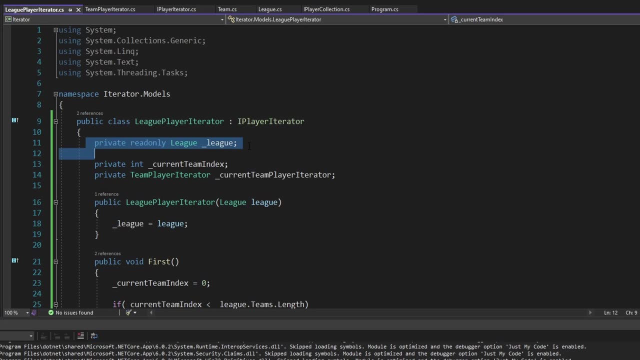 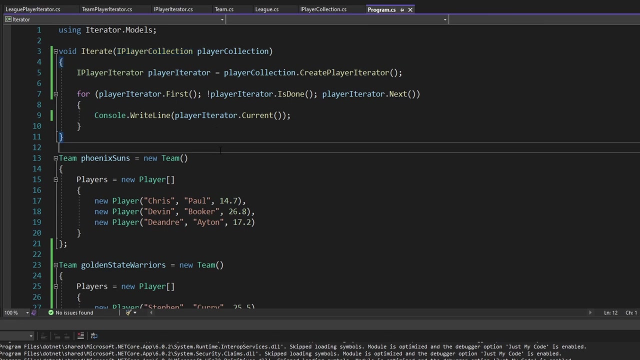 team, it gets back this team player iterator to iterate through the team, And then, if it's a league, we get back this league player iterator to iterate over the league. So now that you know how to create iterators from scratch, you can really apply these concepts to any language. But in C sharp's 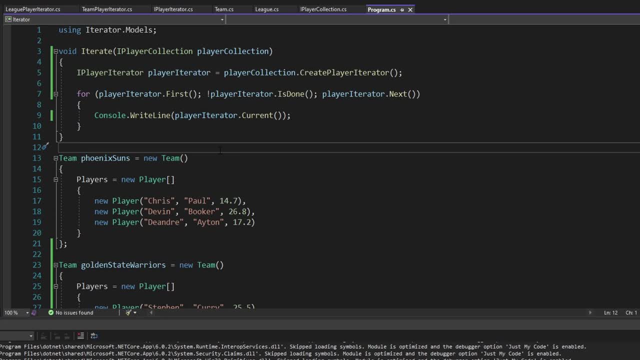 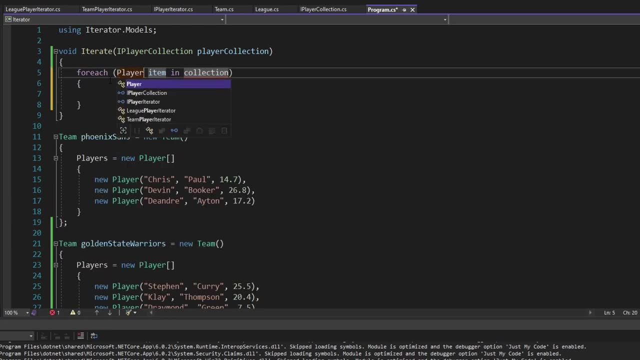 specifically, it's actually much easier to do any of this using yield return. So with yield return, ultimately what we want to do is use a for each and get each player in our player collection and then simply write out that player to the console. But at the moment we can't do this. 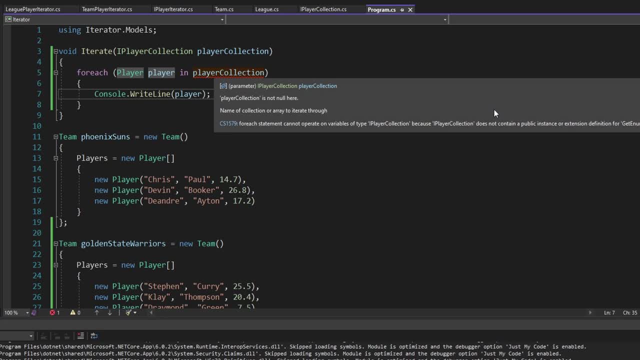 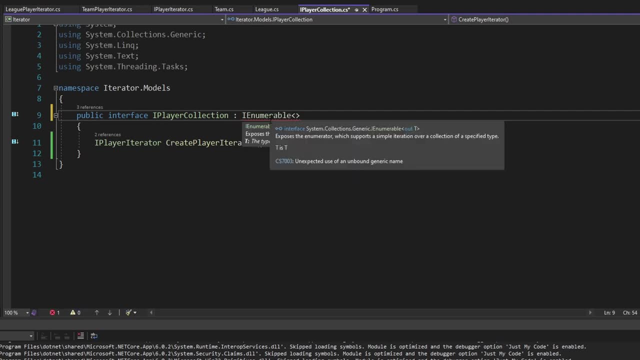 because I player collection doesn't expose a git enumerator function. So if we head into I player collection, we want this to implement I enumerable And we want to enumerate over players. So we want this to be an I enumerable for players And we no longer want to use. 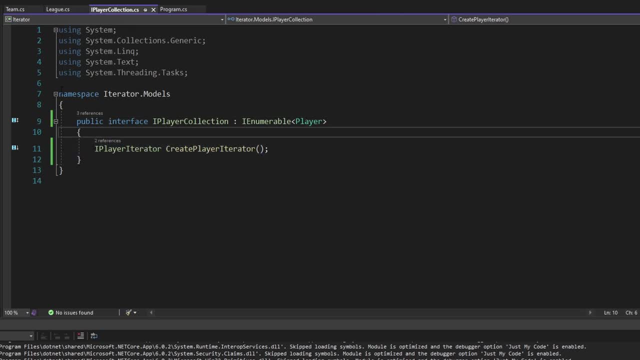 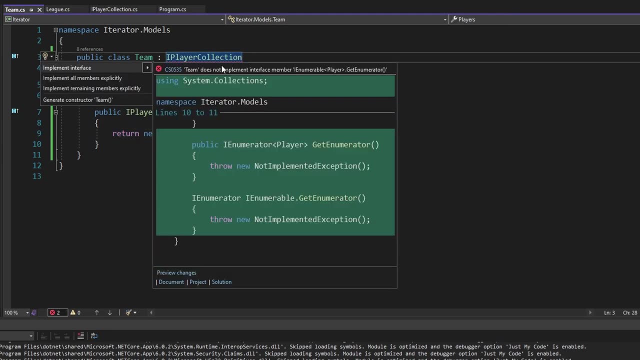 iterators Now, although actually I'll leave it here just so that you can see it in source control. So now back into our team. we want to implement I enumerable for players, So let's implement that interface. So for this non generic function, this is just used to support iteration. 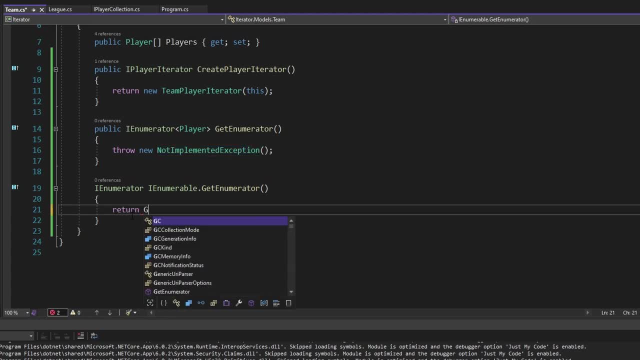 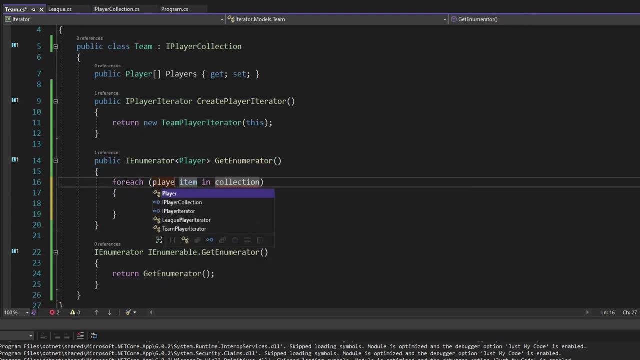 over a non generic array. So for this we can just delegate to the git enumerator function above. And now for git enumerator, we could actually iterate over all the players in our players array and then do a yield return on each player. But in this case, since we're using this players array which already implements- 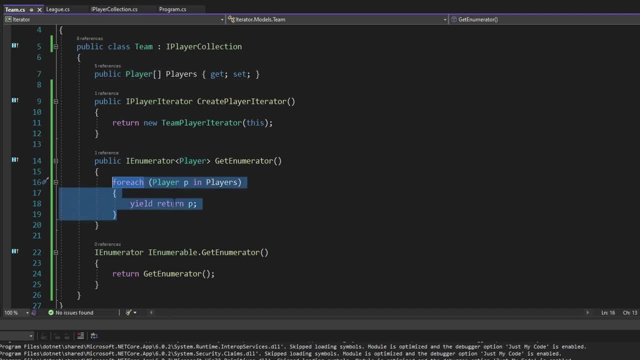 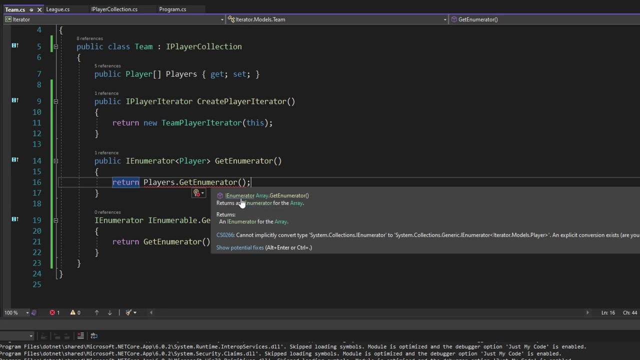 I enumerable. we can just use that here and delegate to it, So we can take our players array and just return its enumerator- Although, whoops, this uses the non generic git enumerator, But in this case we could just convert our players. 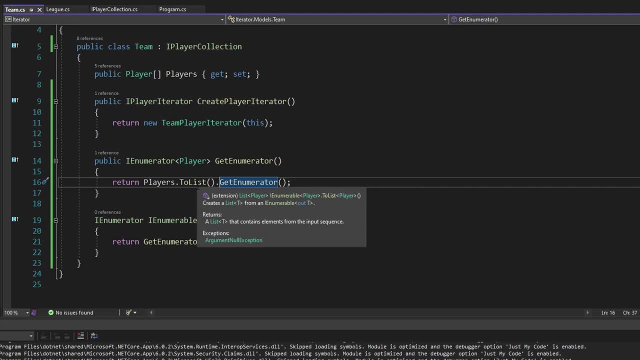 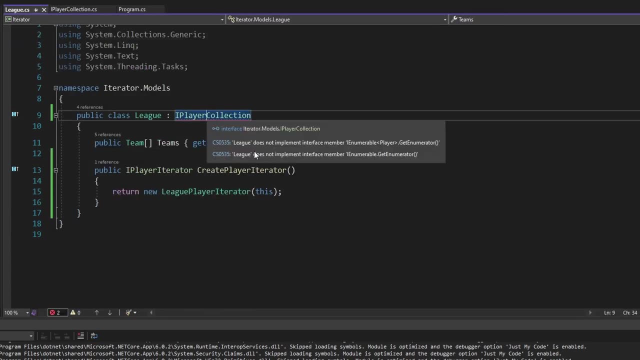 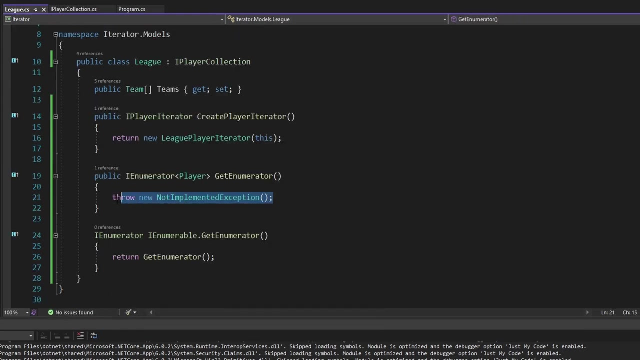 To a list and then call git enumerator on that. And since list is generic, it'll return the generic enumerator as well. So, moving up to league, let's enumerate over this, let's implement that interface And same thing as before: we want to delegate to the generic git enumerator. And now, 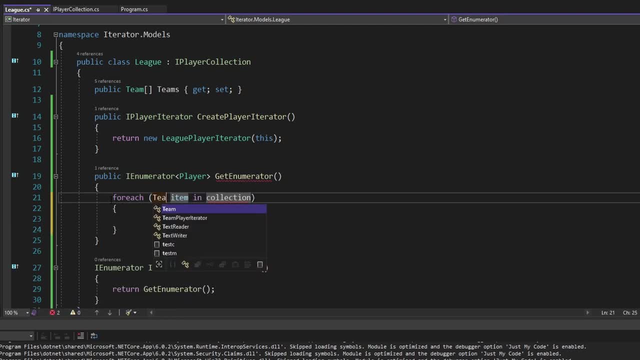 in here we want to use yield return. So first we want to iterate over each team in our team's array and then we want to iterate over each player in the team and then we just want to do a yield return on the player. but basically each time we call yield return on a player, our for each loop. 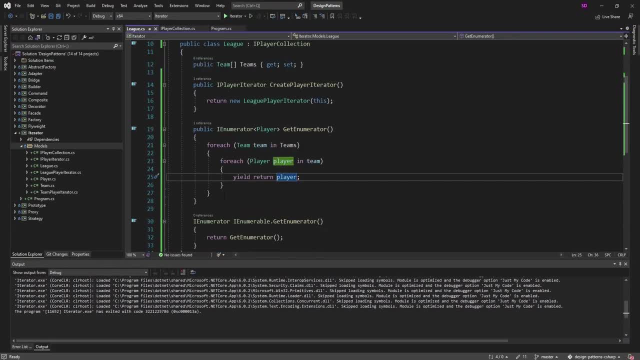 will write that to the console and then, once we're done with all these for each loops, we'll be done with the for each in our iterate function. so let's put a breakpoint here and step through this. so here we go, hitting yield return on our first player and we write that out to the console. 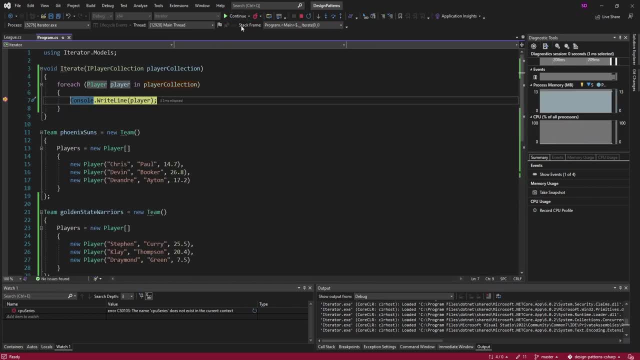 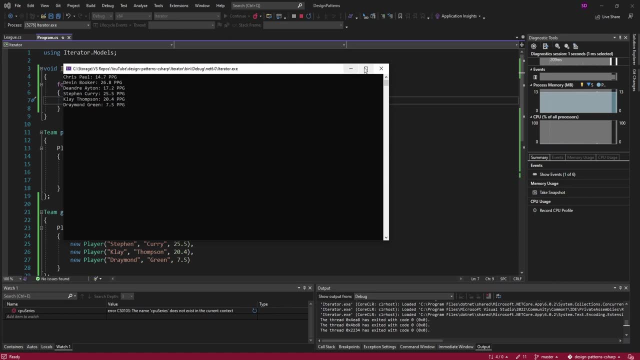 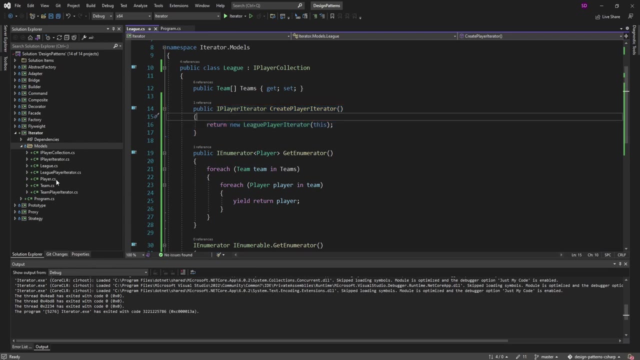 then we continue iterating on to our next player, write that out to the console and so on. so by the end we've still written out all of our players. the difference is that we did not need any of this iterator stuff, so we did not even need the iplayer iterator interface or any of these quirky. 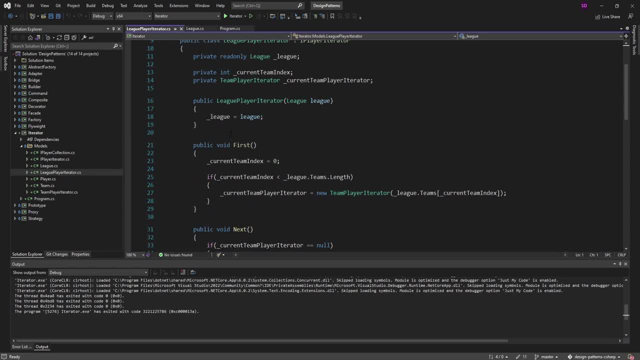 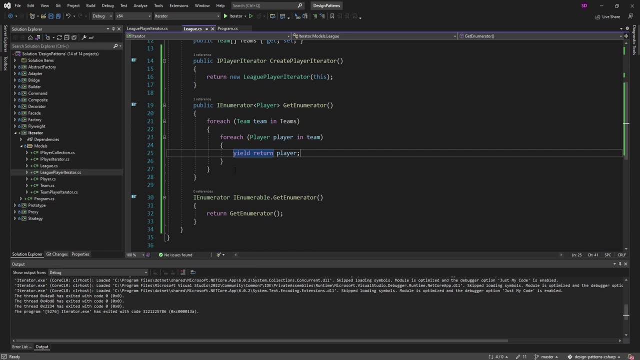 functions and we didn't have to implement an iterator for e e of our different collections. so highly recommend using yield return if you're in C sharp. but aside from that, hopefully you can apply the iterator pattern to your own application so that you can traverse various different collections.